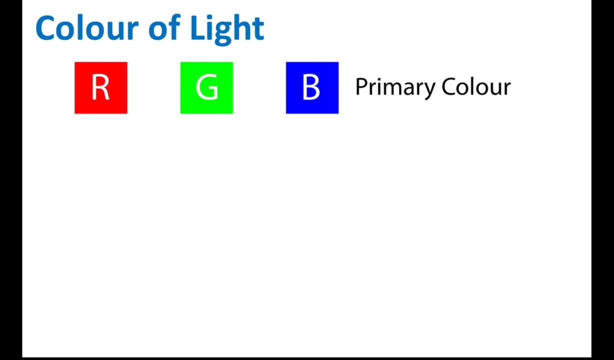 RGB. so RGB are the primary color: red, green and blue. Now, when two different primary colors act together, they will form the secondary color. For examples, when the red colors combine with the green colors, it will form yellow, and when the green combine with the blue, it will form cyan. this is like 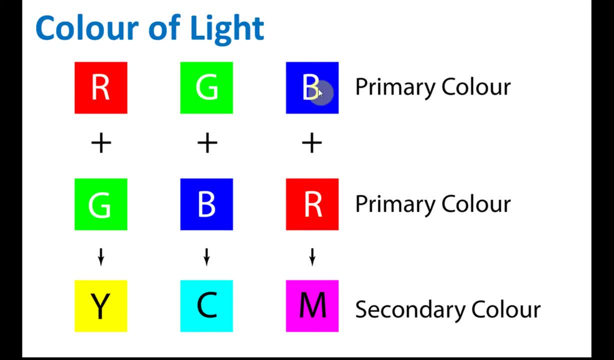 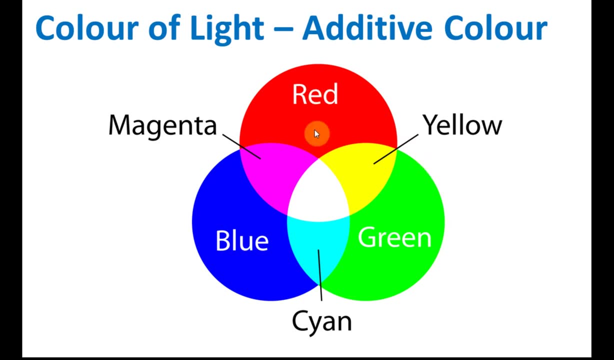 blue is called cyan, and then for blue combined with red, it will form magenta. so this yellow, cyan and magenta are called the secondary color. so this is a summary, okay. so red, green, blue or RGB are the primary color, and red combined with green to get yellow and blue combined with green to 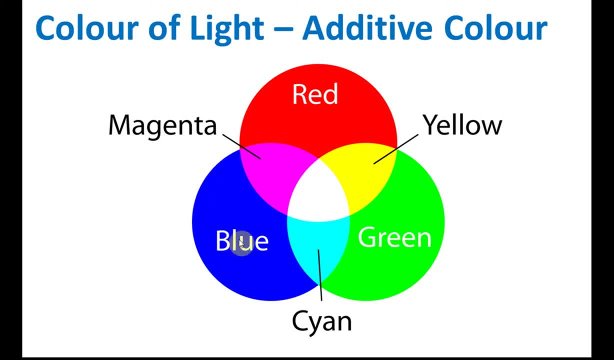 get cyan and red, with blue you get magenta and if all three combines together they will get white. now this is very, very important for you to answer most of the questions, okay? so you must remember this now. let's say, in exam you encounter the questions they ask you about addition and subtraction of color. 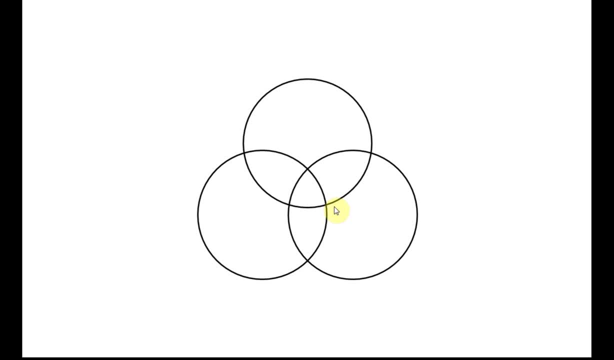 so my advice is: we try to list down all these primary colors and secondary colors. what I advise you to do is draw these three circles, yeah, draw these three circles, and then you can write down the primary colors and the secondary colors and then label it with the color. let's start with the primary color, the 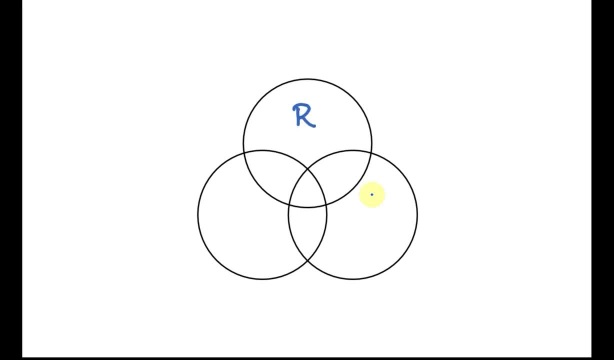 primary colors are the RGB: red, green and blue- okay. after that let's put in the secondary color: red with greens will produce yellow, okay, and red with blue will produce magenta and a blue and greens will produce cyan- okay, and all three combines together will get white. so with these informations, then you 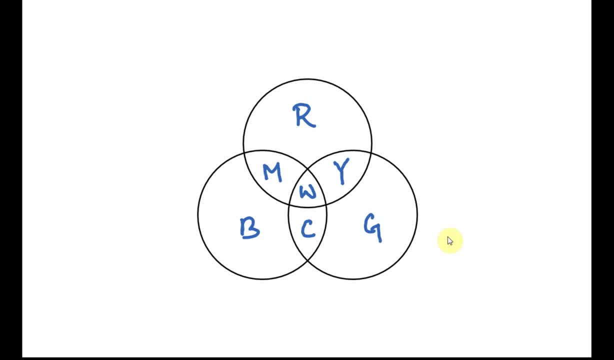 can answer most of the questions easily. so every time when in the example test, you see any questions that related to addition and subtractions of color, then try to list out these informations on a piece of paper and then answer your questions by referring to this information. you.